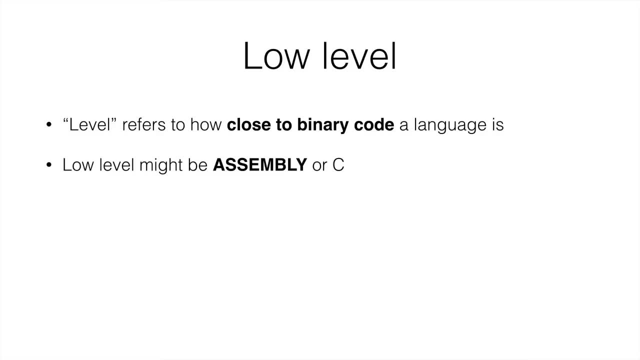 Assembly is a set of instructions that means something in binary. It was used to save programmers time instead of having to write binary code. This means that the code you're about to see can directly translate into binary code. And there we have it. So this is a bit more, a bit easier to read, although you will not directly understand what. 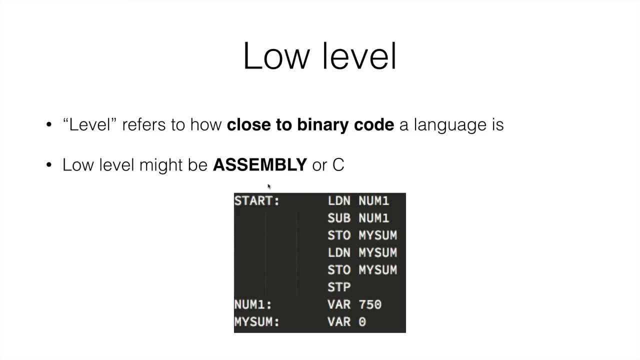 it means- You can see that this is a little bit more complicated than the first one, which is that there's start, where the program is likely going to start, there's a value- 750, if you knew the program multiplies 750 by 2- then this gives you a clue as to what this means. 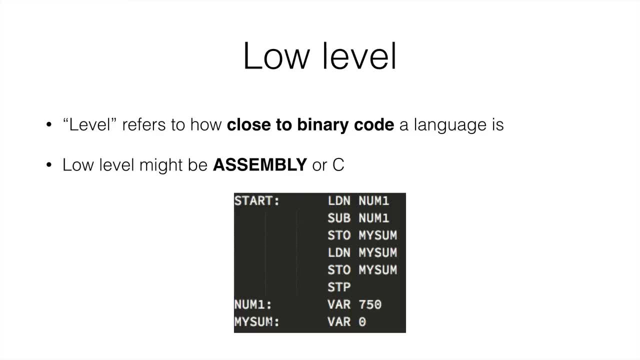 there's num1 and mySum, that if you're English you could see these as potentially two variables or two things that are going to store values, and that's that. so these things you will not understand, but you'll know they refer to num1 and num1 and mySum, mySum, mySum. 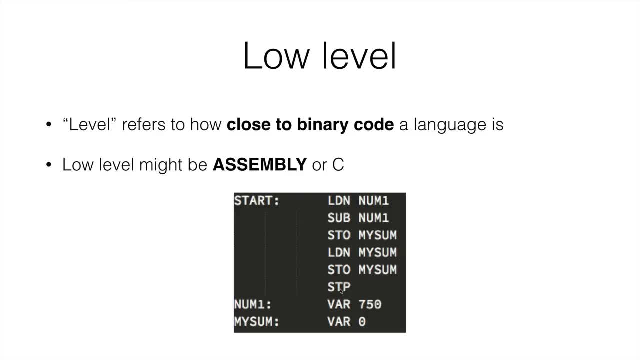 so something is going on here with the variables. stp could stand for stop and it actually does. this ends the program. so it is more readable, but not easy. what I mean with that? it was used to save programmers time and that it means something in binary. I mean that ldn num1. 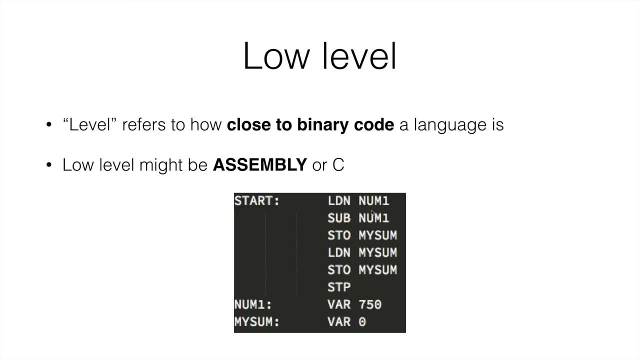 translates to a string of binary code directly. each line translates to one line in binary code. so initially, assembly is low level because it really doesn't do anything for you. it's just: ldn is just a mnemonic for a set of zeros and ones. so let's take a look at what a high level language might look like. 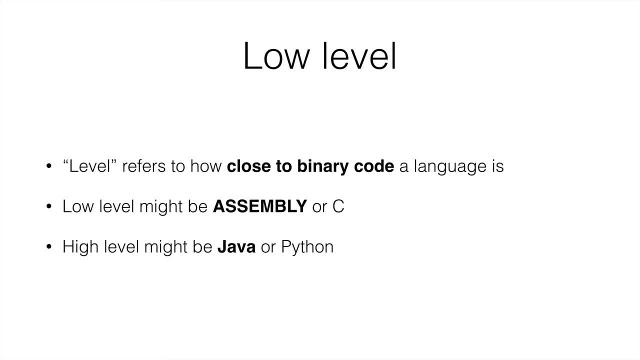 let's take a look at java, which is the language we're going to be learning in this course, and you will see how it is actually a bit easier. this line does the same thing as the whole of the program, and what it does? it creates an integer. 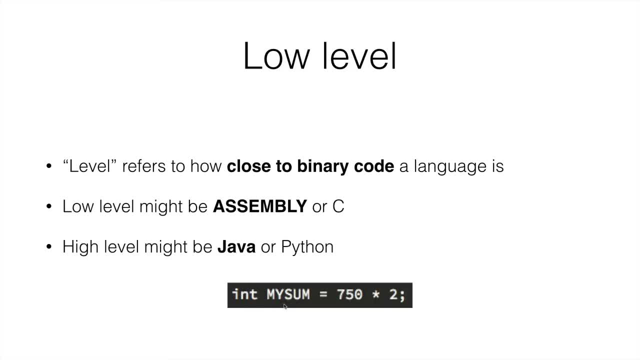 which is a whole number. it calls it mySum. so you have a mySum variable. if you've ever done algebra in mathematics or something like that, you'll see that mySum is just a variable of type integer, which means it can only hold a whole number. 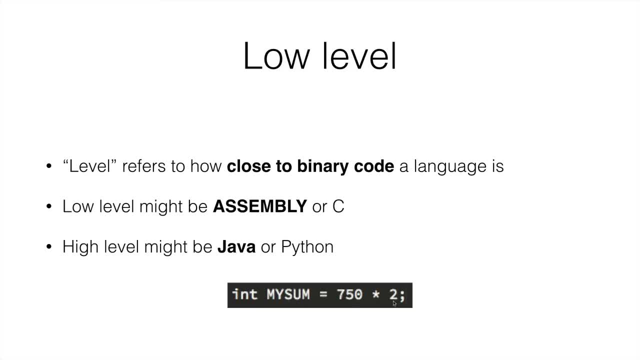 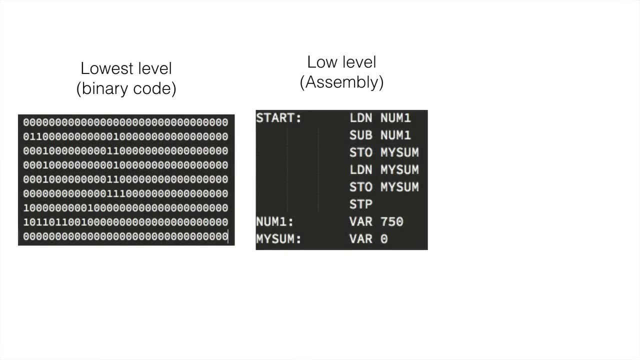 and then this equals 750 multiplied by 2, so you create an integer variable called mySum that holds a value of 1500, and this does the same thing as the other program does. ok, so we have binary code, we have assembly, and then we have java. 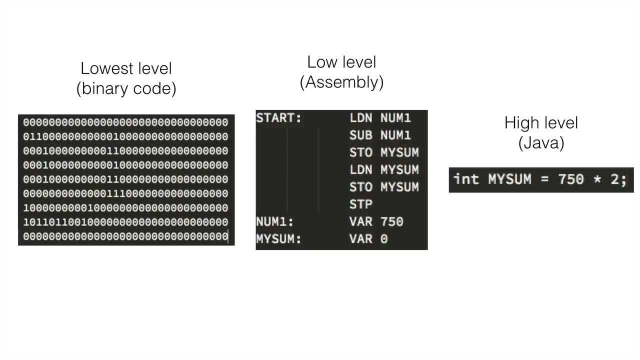 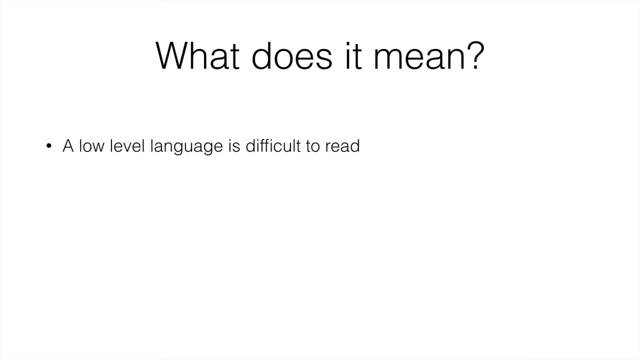 and, as you can see, they get easier over time. so what does it mean to be a low level language? a low level language is difficult to read, whereas high level languages are more abstract and they do things for you and also contain natural language elements, for example java, the language we will be learning in this course. 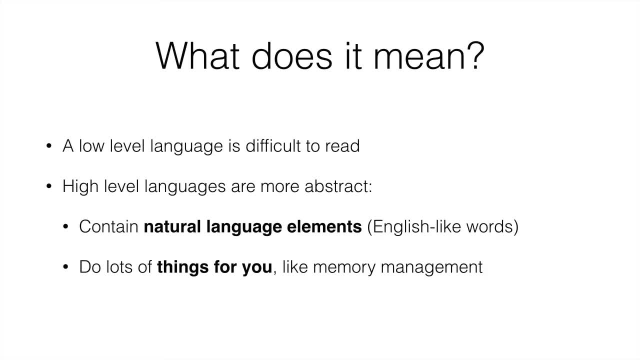 contains many english words that make it easier to read and easier to understand. in addition to that, I said that they do lots of things for you. what I mean with this is that those binary and assembly languages were so long because you had to tell the processor when to stop doing things. 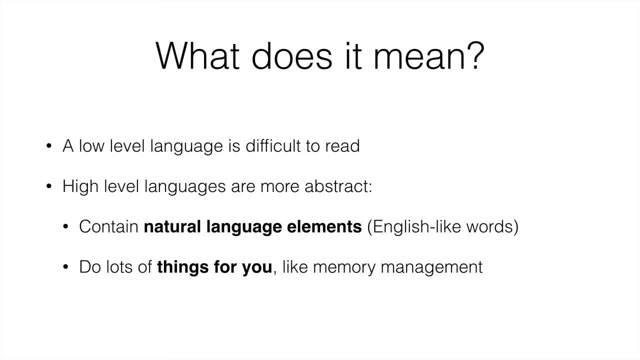 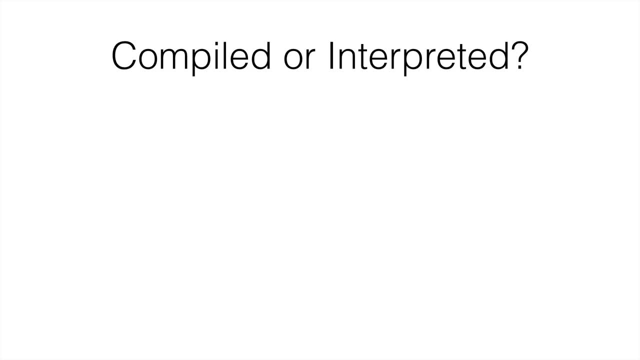 you had to tell the processor where to get the data from. in java it takes one line because it does all of that for you. and then the other grouping is whether languages are compiled or interpreted. so there are two main types. and compiled languages are compiled and interpreted. 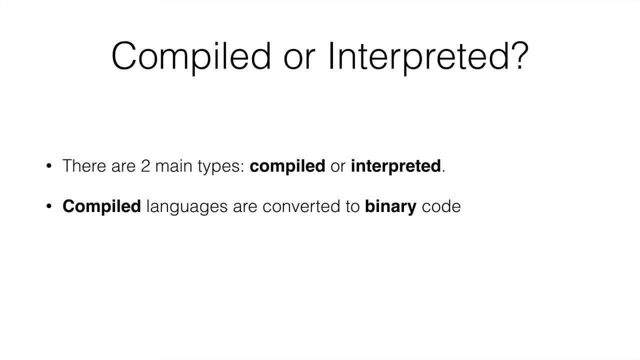 compiled languages are converted to binary code directly. this means you get the source code, for example in a language called C++. you run it through a program called the compiler and out comes binary code, zeros and ones. the computer can only understand binary code. so this is perfect. you give the computer the binary code. 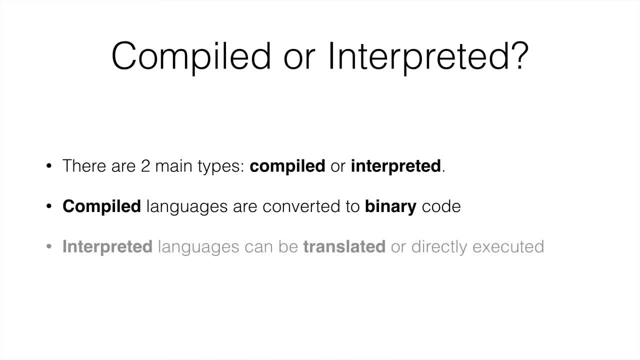 and then it runs through it really quickly. interpreted languages can be translated into a different language or directly executed. what I mean with this is that you'll get your source code in an interpreted language and you'll have to run that source code through a program, and this program will communicate with the computer and with the processor. 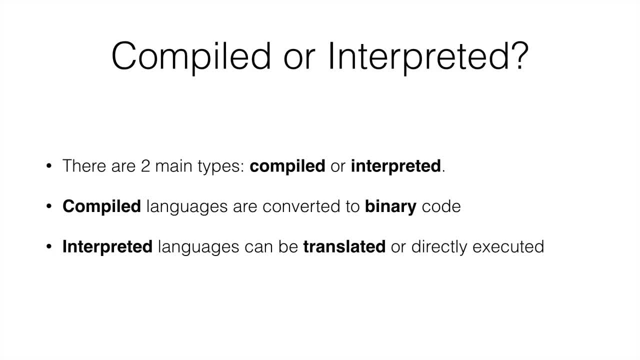 your code doesn't get converted into binary code directly. this is slower because you're depending on a program to communicate with the computer and not giving the computer the instructions directly. so why would you want to use an interpreted language? well, I'll come to that in a second, when we talk about the language we're going to be learning. 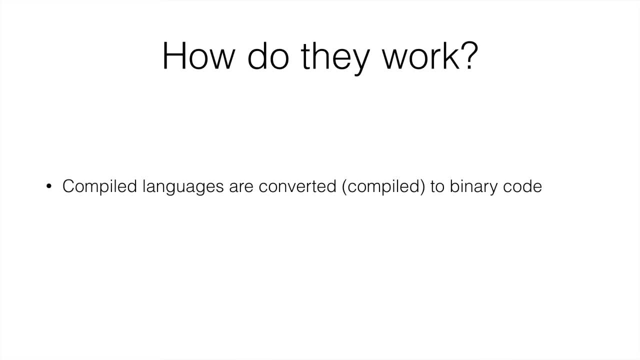 so how do they work? compiled languages are converted or compiled to binary code, and the computer can then run this binary code, as we've agreed. so it's something like this. it's fairly simple: you get your source code, you give it to a compiler. 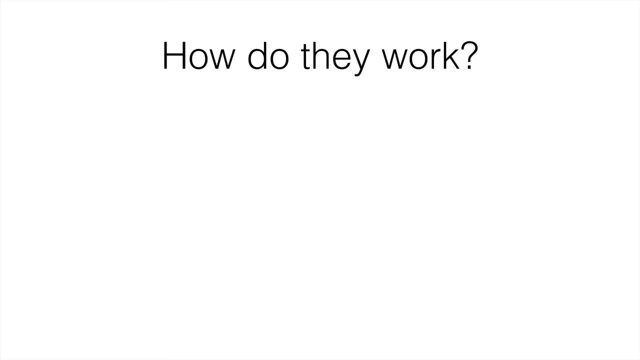 you get binary code and then you give it to the actual computer. interpreted languages are run by a program that interacts with the computer. and this extra step, the interpreter, this program that interacts with the computer instead of giving the binary code directly to the computer. that makes interpreted languages slower. 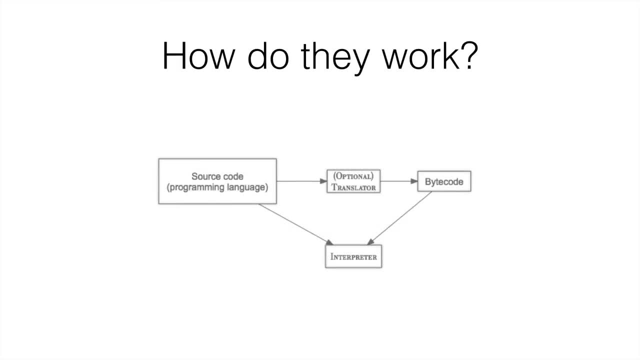 because you're depending on another program and it goes like this: you get your source code at the top left and then you can translate it into a simpler language or you can directly interpret it. it's up to the program's design and then you interpret that. Java, in our case, is the language we're going to be learning, and Java is translated into bytecode. 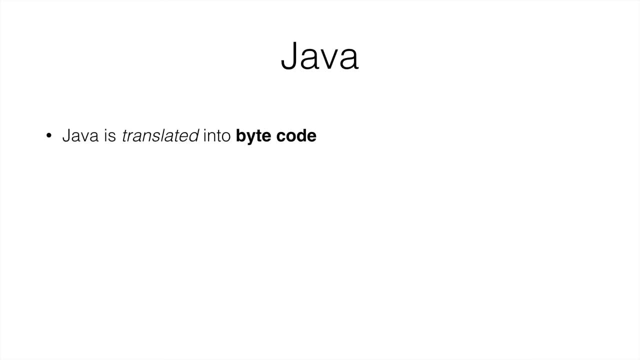 you do not have to learn bytecode or anything like that. we will only learn Java in this course, and this makes it easier to to interpret. and this bytecode is uninterpreted. the program that interprets this is called the Java Virtual Machine. Java Virtual Machine is a program that is installed in many computers and many other devices. 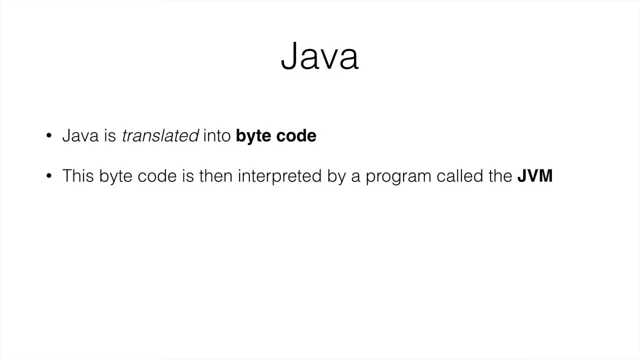 for example, your Android phones or your Mac or Windows or Linux. all those computers have the Java Virtual Machine, usually by default, and this means it comes installed with your system, so all those systems can run your Java programs. however, Java is a fairly slow language because of this. 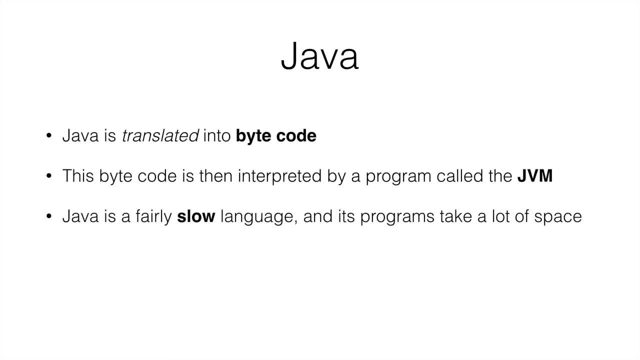 because it has this interpreter and it needs it. Java is fairly slow compared to at least other compiled languages, and also Java programs take a lot of space. what i mean with this is that when you send someone your program, you're not actually only sending a program, you're also sending a lot of the Java language that your program depends on. 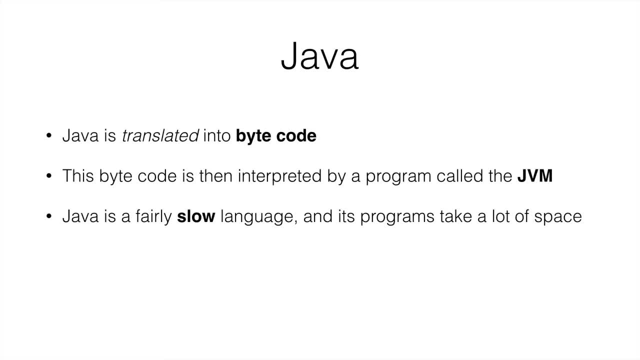 and that the Java Virtual Machine needs and things like that. so you're actually sending quite a large chunk of data when you send someone a Java program. that's why Java programs take a lot of space. however, the benefit is that Java is fully portable. you write your Java program in your Mac. 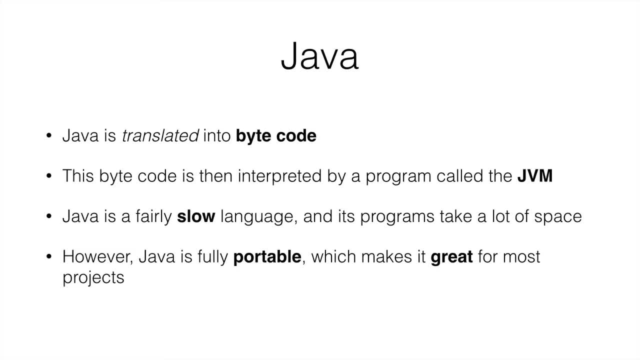 and then you can run in Windows, Linux, Android or anywhere you want, and this makes Java brilliant for many projects and this is why we're using it as well. the things I write here on my Mac, you write the same in your Windows computer and it just works.